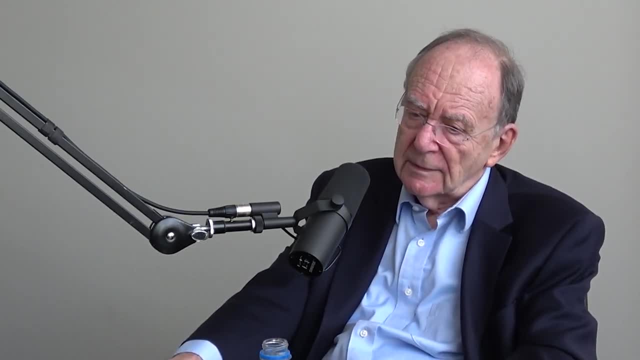 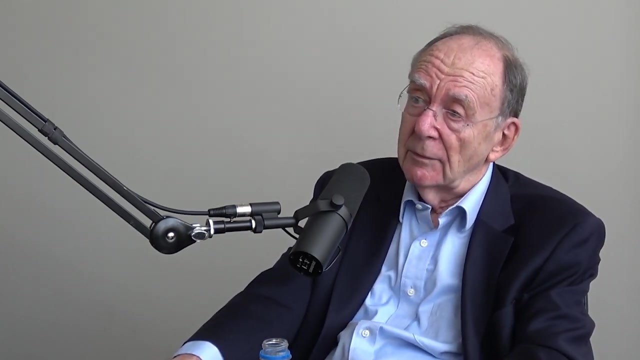 If you had to bet all your money on it, I would bet that P is unequal to NP, simply because there are problems that have been around for centuries and have been studied intensively in mathematics, and even more so in the last 50 years since the P versus NP was stated, And no polynomial time algorithms. 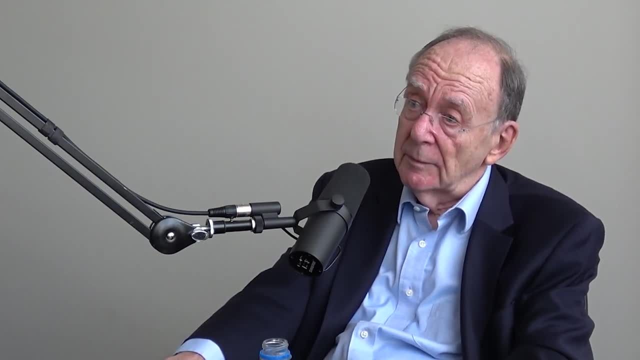 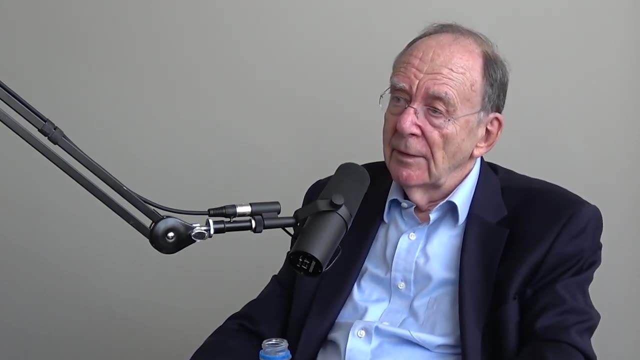 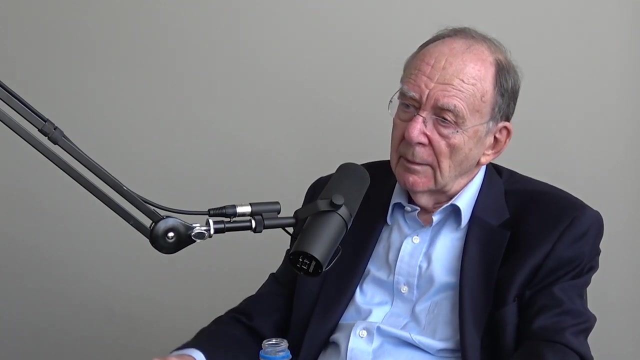 have been found for these easy-to-check problems. So one example is a problem that goes back to the mathematician Gauss, who was interested in factoring large numbers. So we know what a number is prime if it cannot be written as the product of two or more numbers. 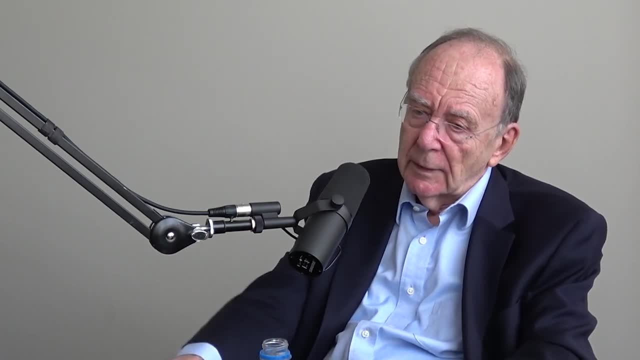 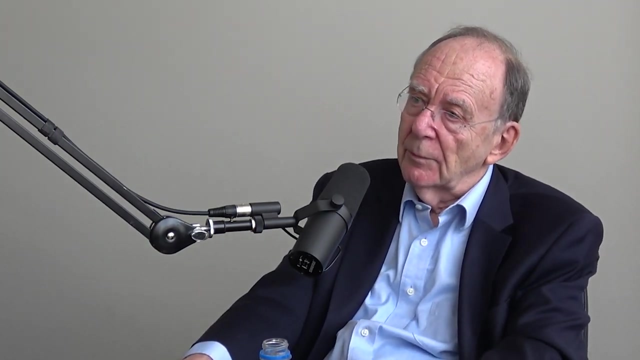 unequal to one. So if we can factor a number like 91, it's 7 times 13.. But if I give you 20-digit or 30-digit numbers, you're probably going to be at a loss to have any idea whether. 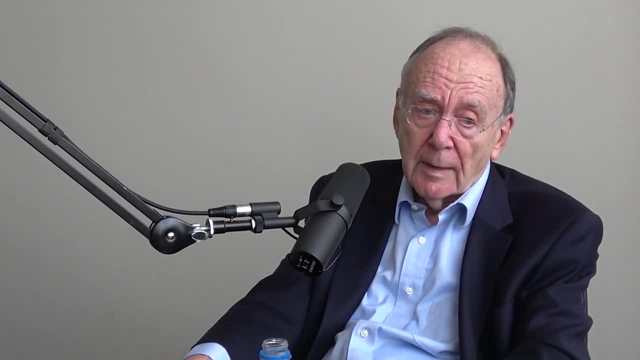 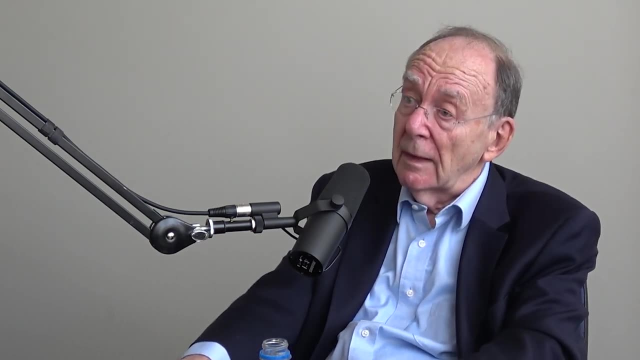 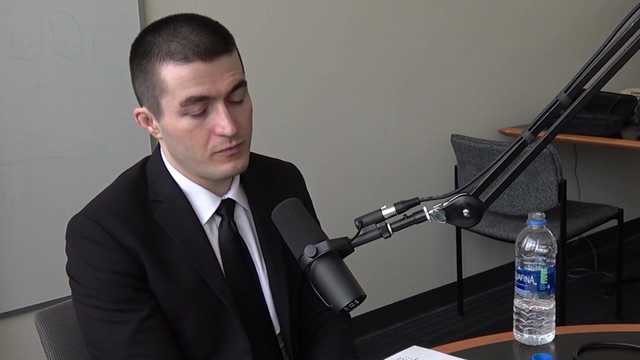 they can be factored. So the problem of factoring very large numbers does not appear to have an efficient solution. But once you have found the factors expressed the number as a product of two smaller numbers, You can quickly verify that they are factors of the number. 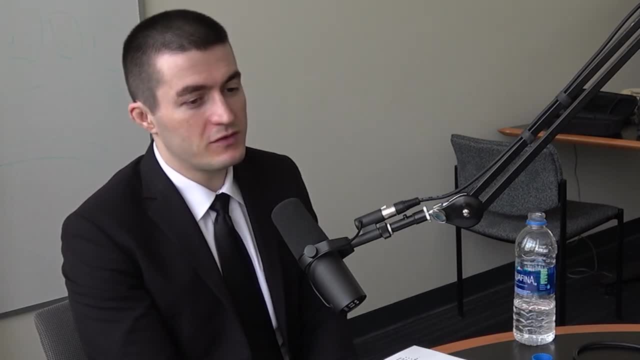 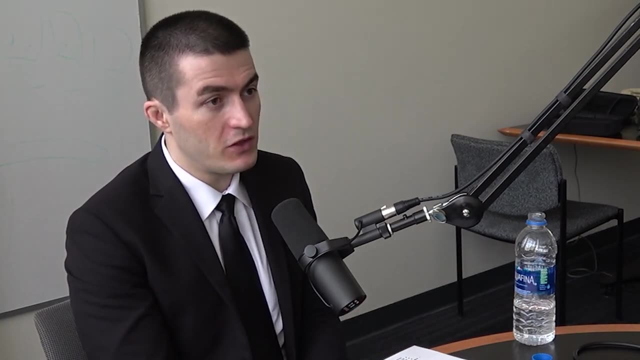 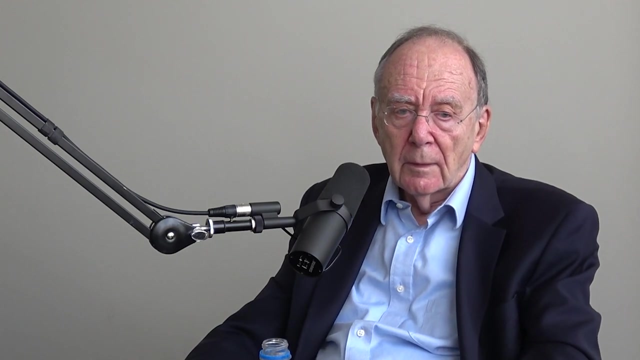 And your intuition is. a lot of brilliant people have tried to find algorithms for this one particular problem. There's many others like it that are really well studied, and it would be great to find an efficient algorithm for Right And in fact we have some results that. 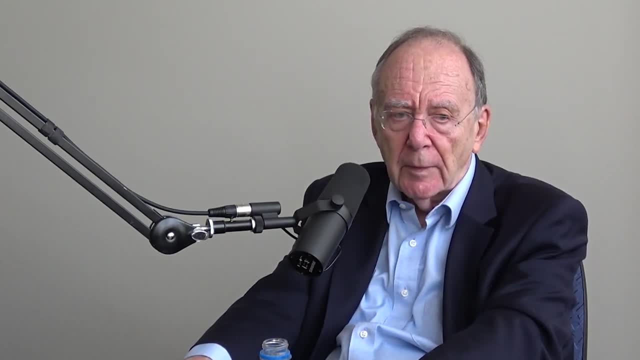 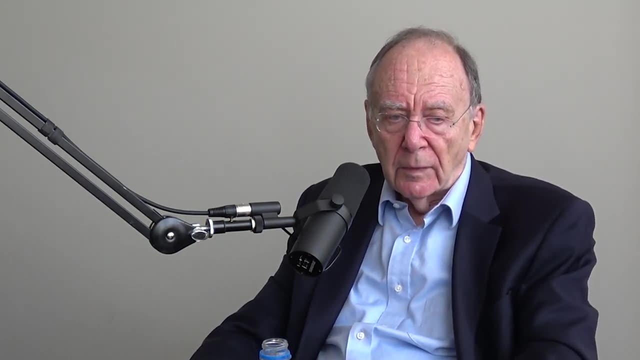 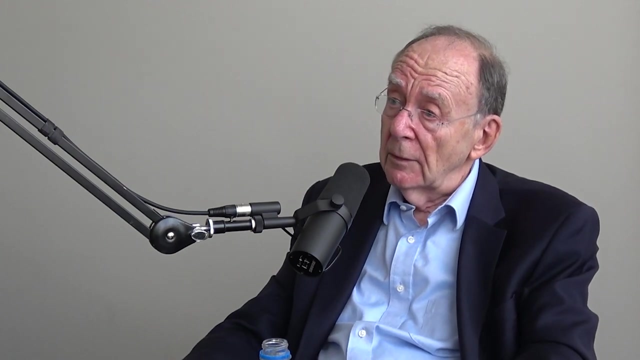 I was instrumental in obtaining, following up on work by the mathematician Steve Cook, to show that within the class NP of easy-to-check problems, there's a huge number that are equivalent in the sense that either all of them or none of them lie in P, And this happens.